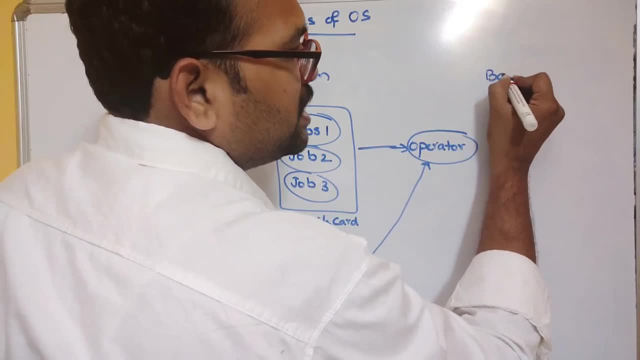 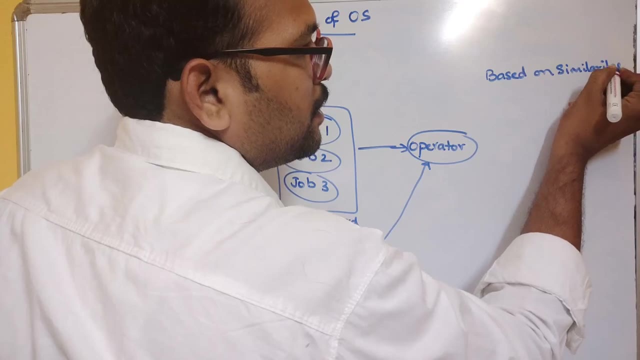 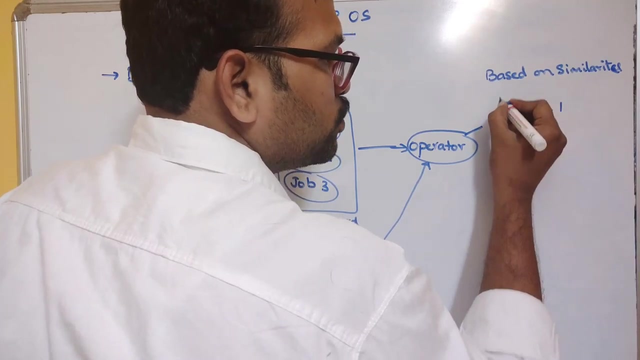 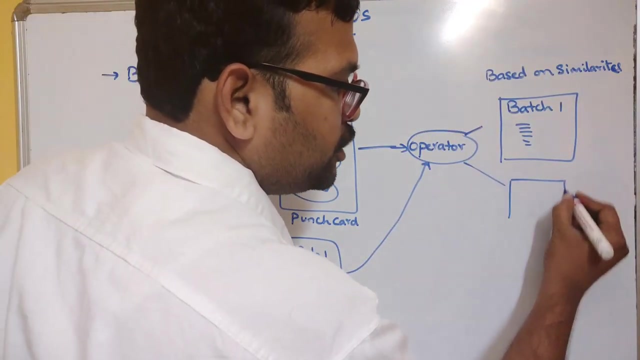 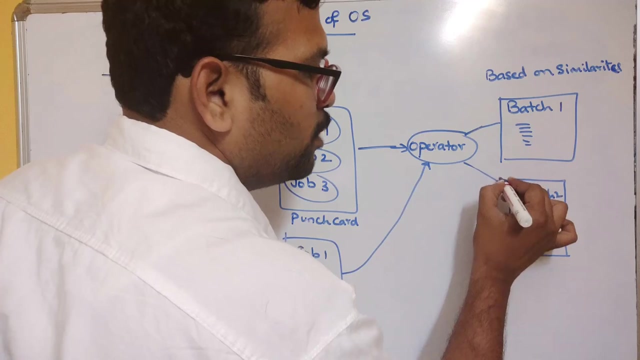 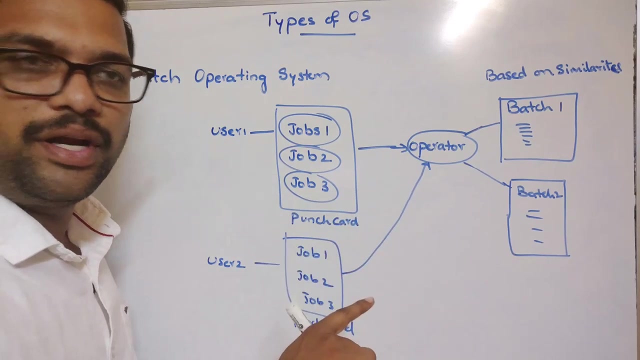 So, based upon the similarities, based on similarities, this operator will create a batches Batch 1.. So batch 1 will be having different jobs with a related similarities. Similarly, batch 2. Batch 2. Okay, Okay, So it will be having a different jobs with a related similarities. So this is how the programs will be executed in this particular batch operating system. 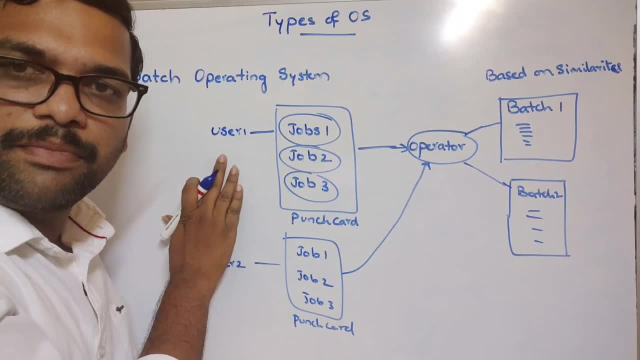 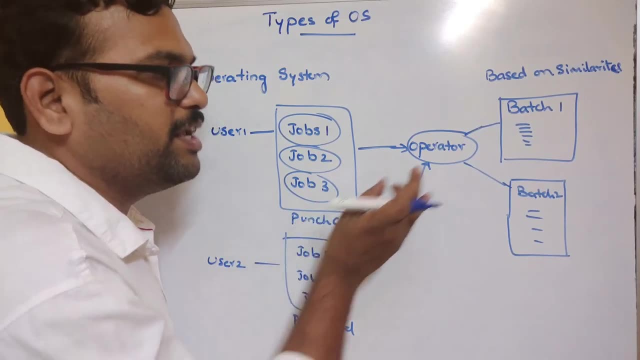 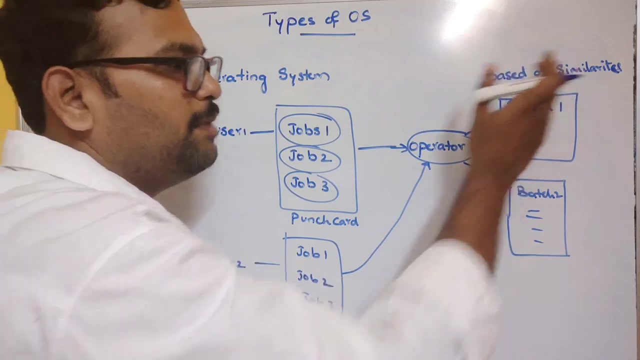 So user will not be communicated to the system directly. So the user will create the jobs and it will be placed in a punch cards and these punch cards will be given to the operator. So operator will collect the different punch cards from different users and, based upon the similarities, the operator will collect the different punch cards from different users. 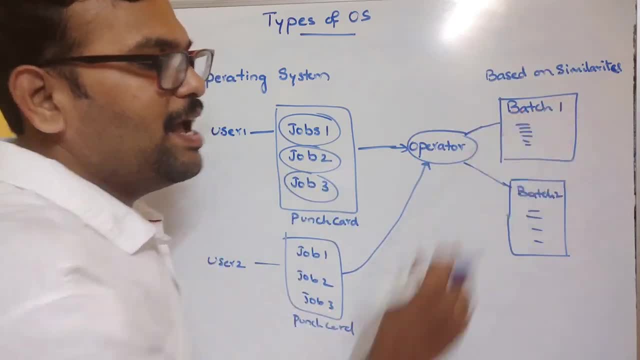 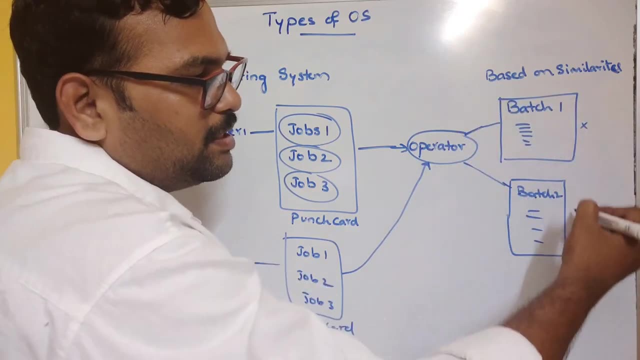 So an operator will group the jobs and we call them as batches, And at a time one batch will be given to the CPU right, And here the drawback is, until the batch 1 completes this, batch 2 will have to wait. Okay. 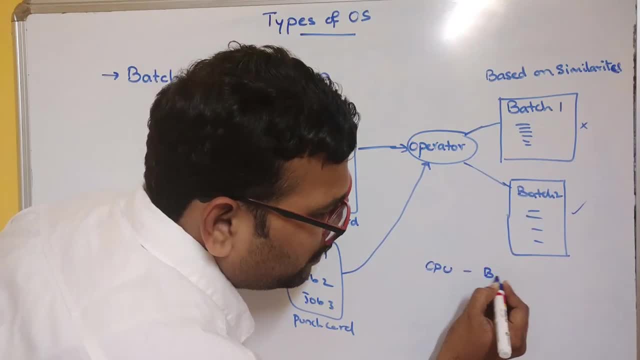 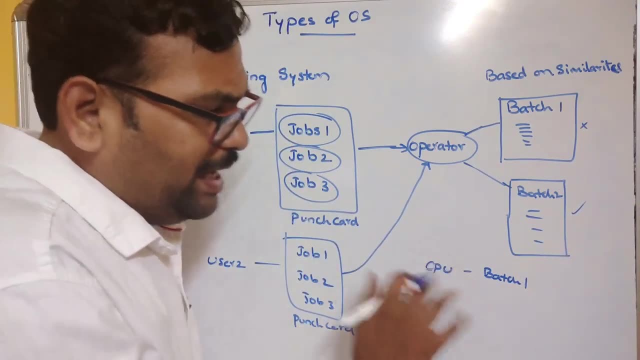 Until the CPU completes the batch 1, okay, The batch 1, batch 2 jobs should be in a waiting position. So, even though so here the main drawback is CPU utilization, So if the CPU may be in ideal state, Okay, Okay. 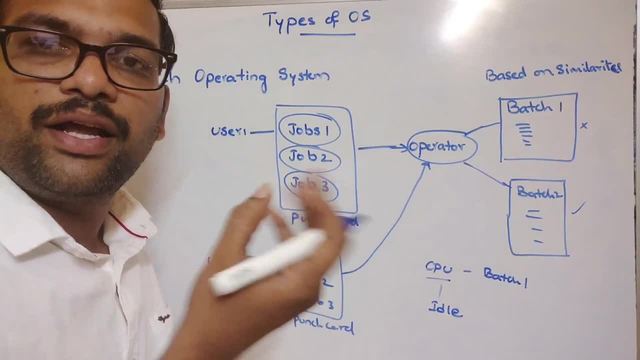 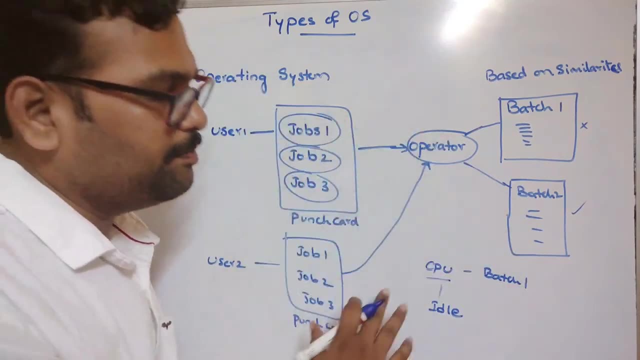 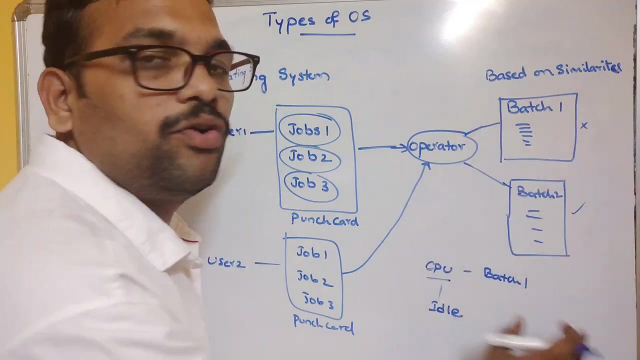 CPU may be in an ideal state. If any process is requiring the Ivo operations, then the CPU have to wait until it completes the Ivo operation, and after that only the CPU can execute the processes. So until the batch 1 completes the batch 2 and again batch 2 completes, then only batch 3.. So 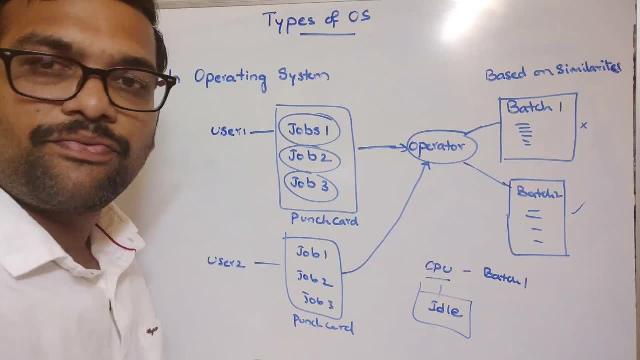 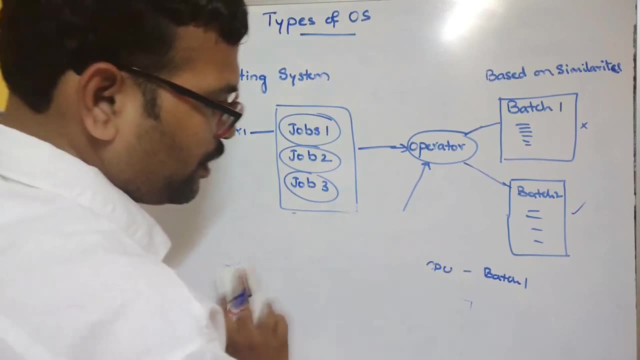 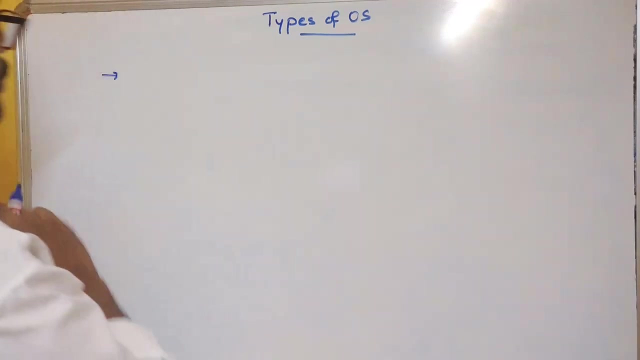 there might be a chance of ideal idleness of a CPU. So this is about our batch operating system. So, coming to the second one, in order to reduce the CPU, ideal time, in order to reduce the CPU, ideal time. the second one is multi-programmed operating system. So here the name itself. 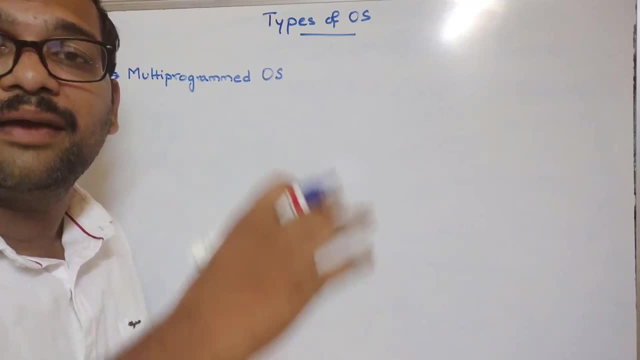 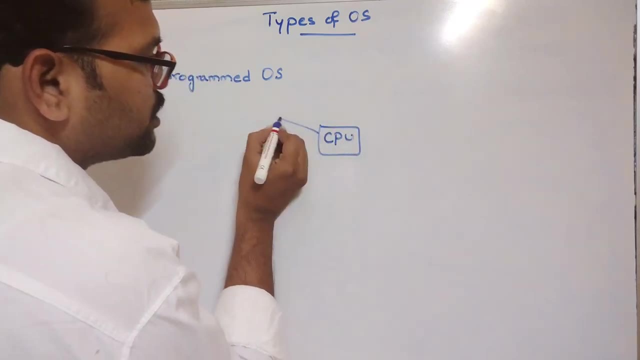 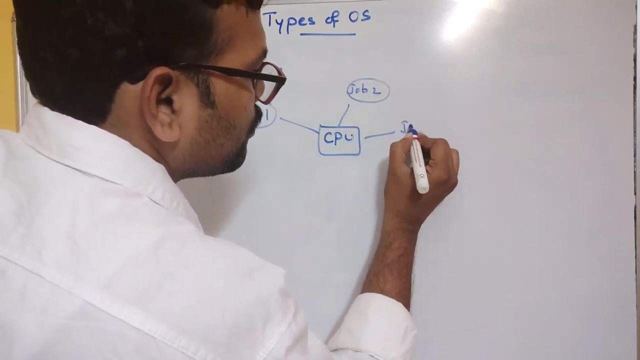 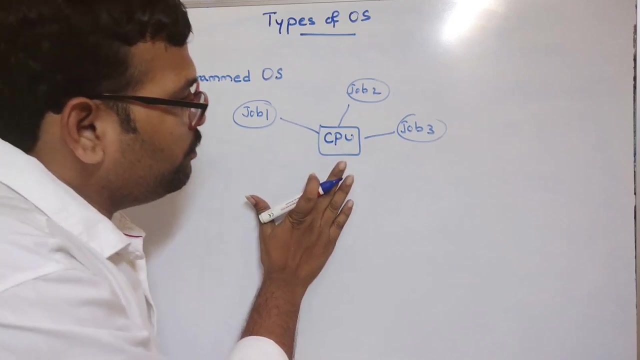 indicates multiple programs will be given at a time to a CPU. So if it is a CPU, then multiple programs. so job 1, job 2, job 3, right, So multiple processes will be given to the CPU, so that so CPU first executes the job 1 and if this job 1 requires any Ivo. 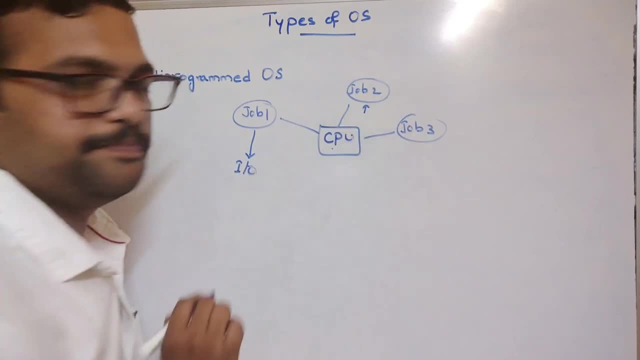 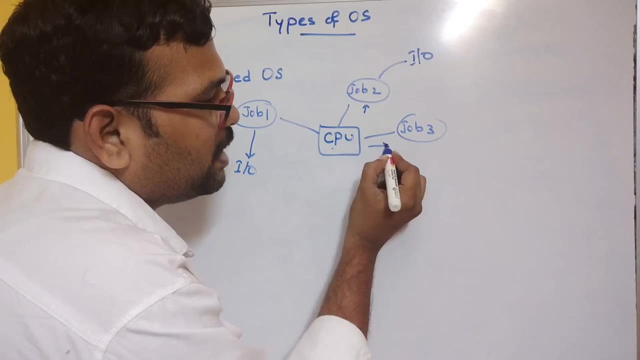 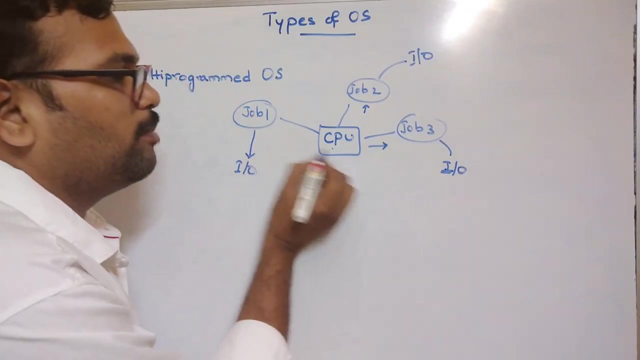 immediately the CPU will start executing this job 2.. So if the job 2 is also required, some Ivo operations, immediately the CPU will start executing the job 3.. And still the job 3 requires any Ivo operations, immediately again CPU will be start resuming the. 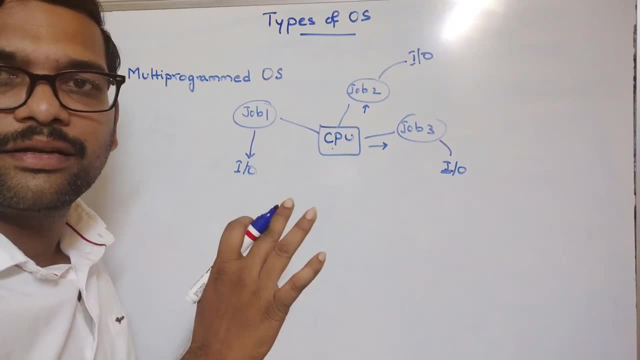 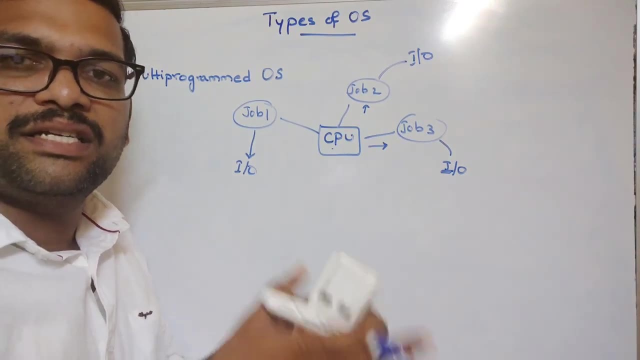 job 1.. So that means there will be no ideal stage for the CPU. CPU will not be in an ideal stage, So CPU will be switching between the processes based upon the Ivo operations. right. So CPU doesn't go to the ideal stage, So CPU will be switching between the processes based upon the 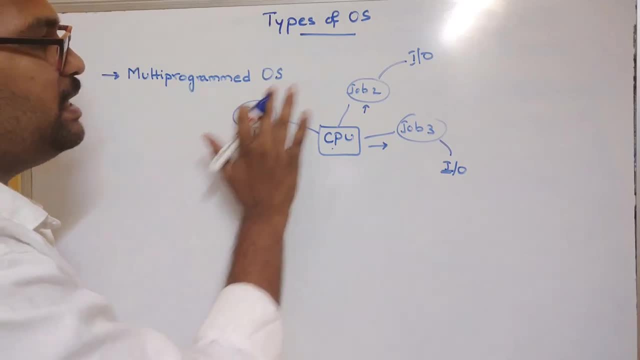 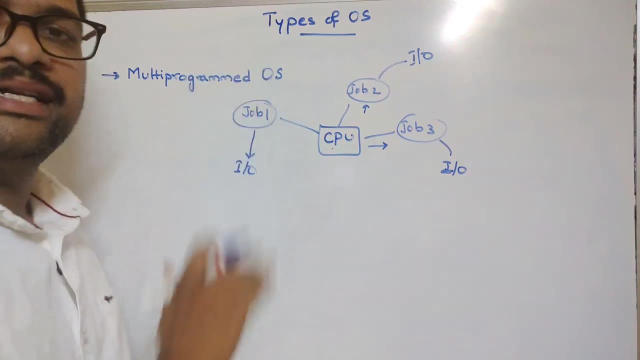 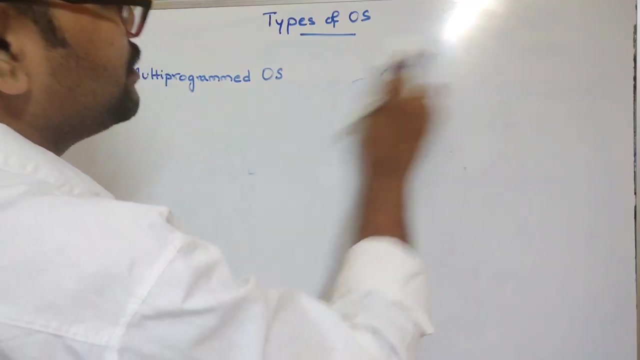 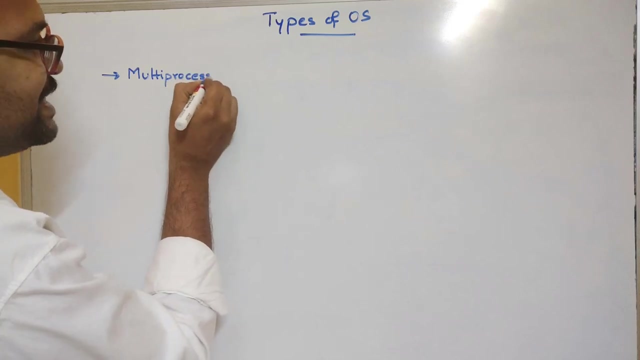 ideal position. So here you can see a multiple programs are executing at a time by the CPU, So that's why we call it as a multi-programmed operating system. multi-programmed operating system. right Next. the next category is multi-processing operating system- multi-processing operating system. So, coming to this multi-processing 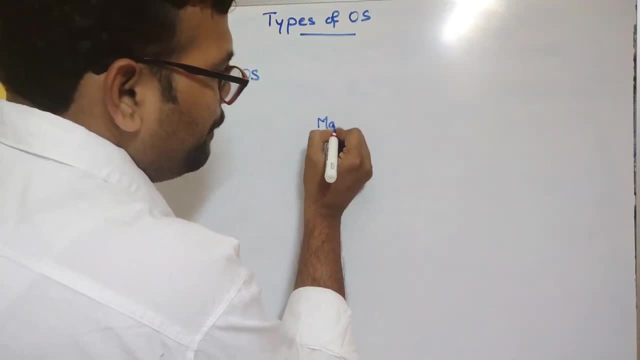 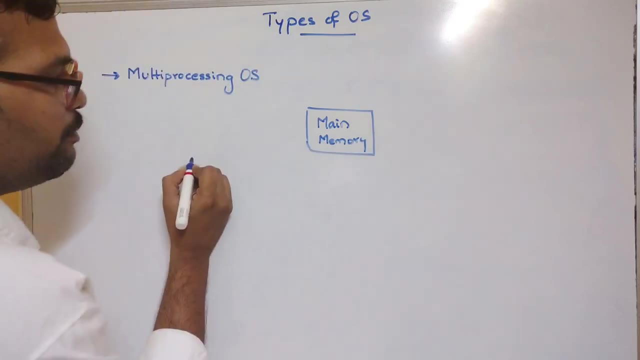 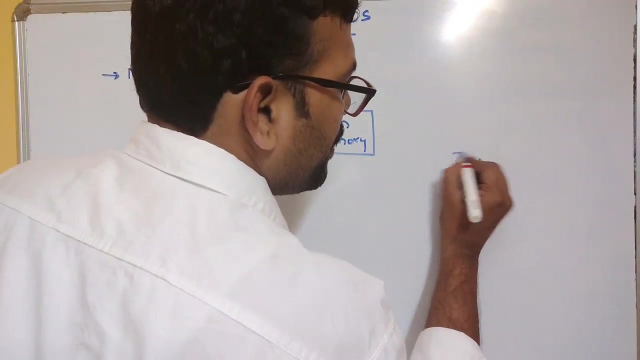 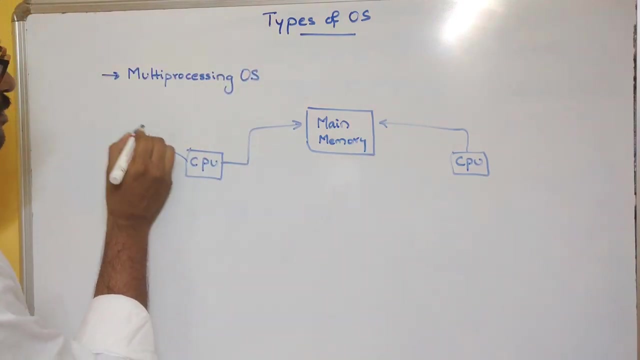 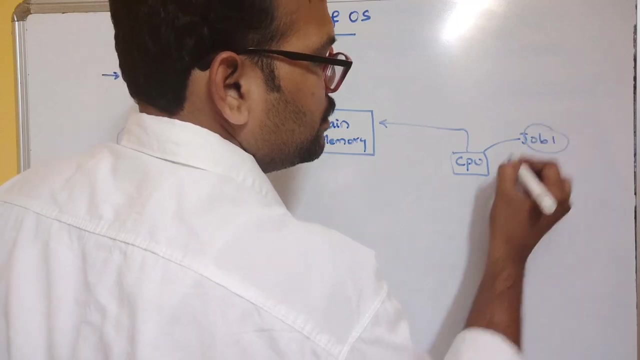 operating system. so a memory will be there and there will be a different processors. There will be a different processors accessing the memory. So at a time, multiple processes: okay, Job 1, job 2.. Similarly, in Ivo, Ivo, OMG works for here. So here the multiple processors will. 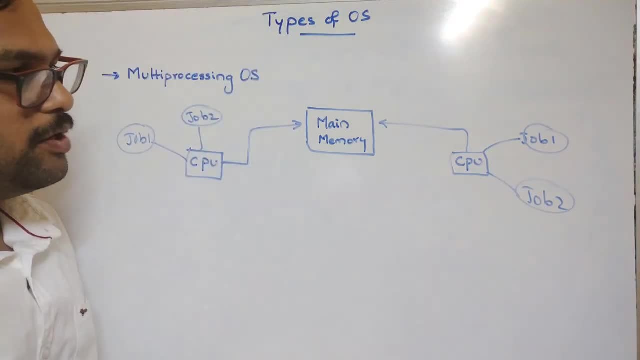 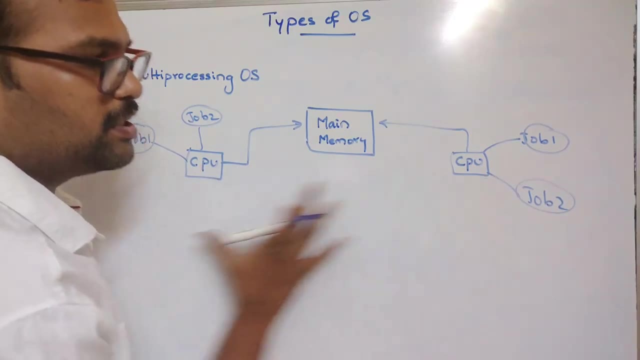 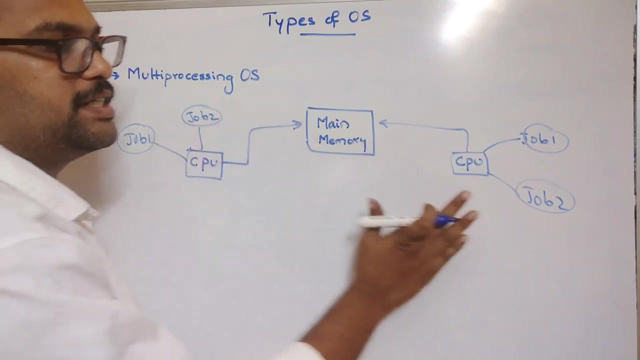 be having will be connected to the same computer, multiple processes using the multiple processors. Okay, So here we are having two processors and the jobs are divided between two processors. Okay, So here the CPU will execute the job 1,, job 2, and CPU will be execute the job 1, job 2, but both the processors are connected to the same system. I can see herely, or rather weiß peninsula有人. productivity performance. in the Ivo icher system where aye two brotherss can go to work together, That means the CPU will run the job. 1-2. Vocאלyorum i 제품. tid looks simultaneously running over. addition to that, t ane you. 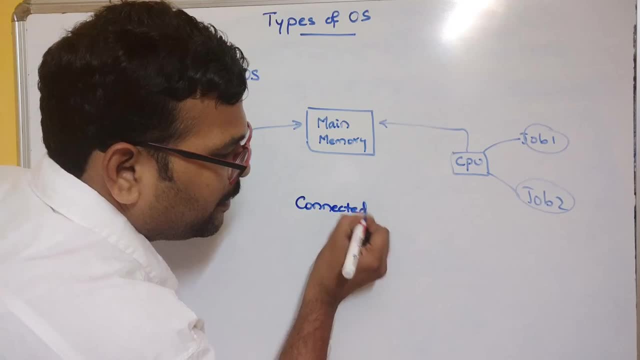 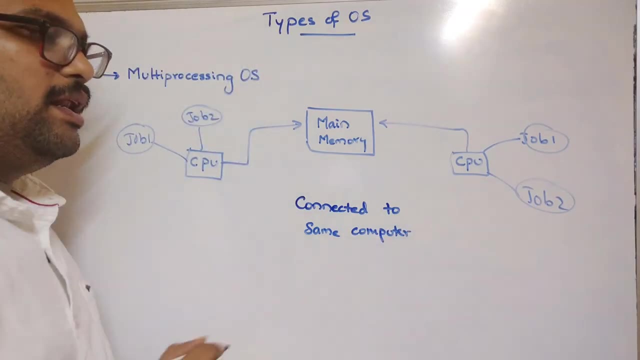 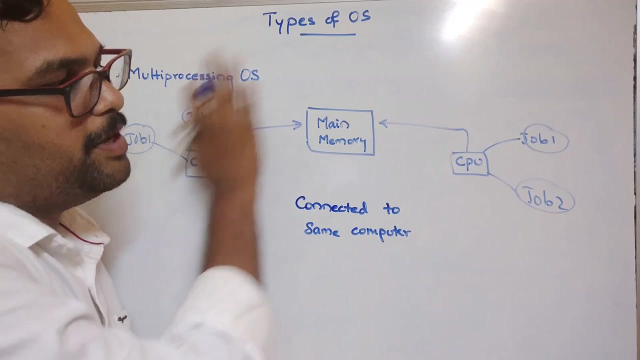 same system, so connected to the same computer, same computer, so automatically. so the jobs will be shared right. so easily and fast we can execute the jobs. so one more thing: if any one of the processor fails, automatically the jobs will be executed by the another processor. so this is the main advantage. 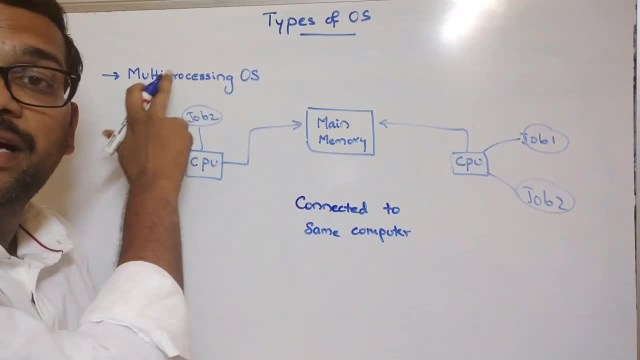 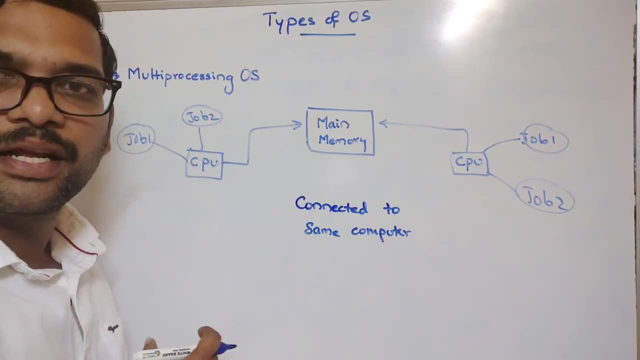 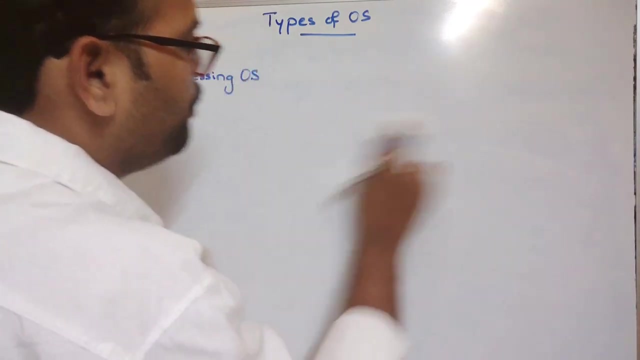 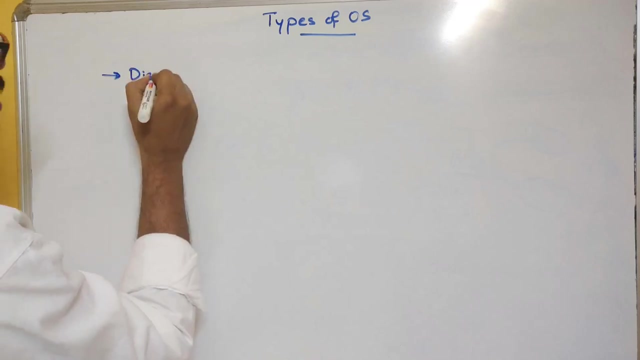 of using this multi processing, so the name itself indicates. multi processing means multiple processors will be connecting to the same computer and the programs will be get executed right. this is the next one. we will move on to the next one. next type of operating system: distributed operating system. 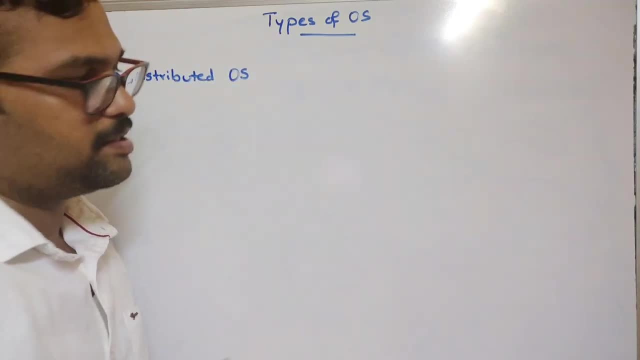 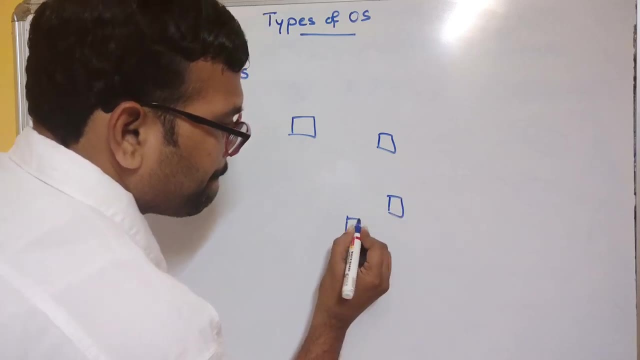 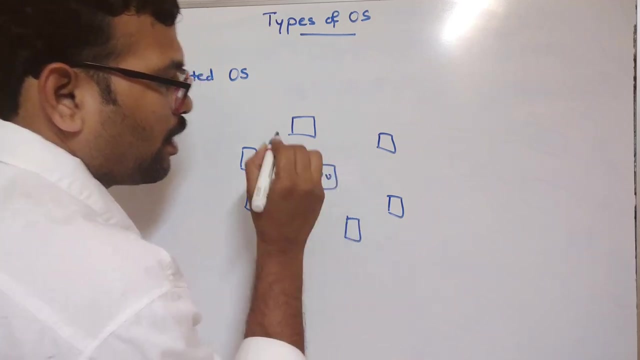 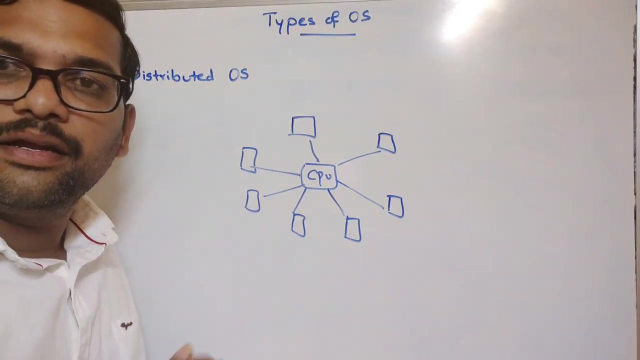 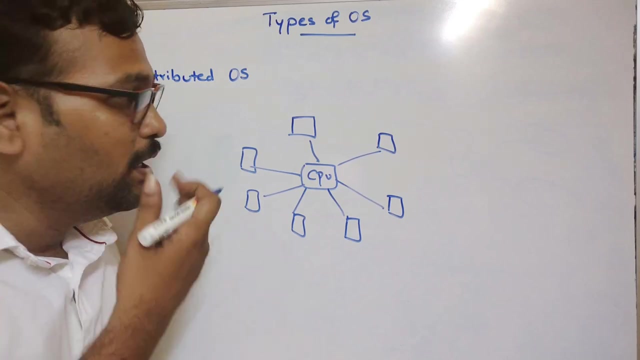 distributed operating system. distributed operating system, so also we can call it as a network operating system. so there will be a lot of computers connected. okay, so here the jobs will be distributed by the different processes, the jobs will be distributed to the different processes, so at a time we can execute the multiple processes. okay, multiple processes, and see. 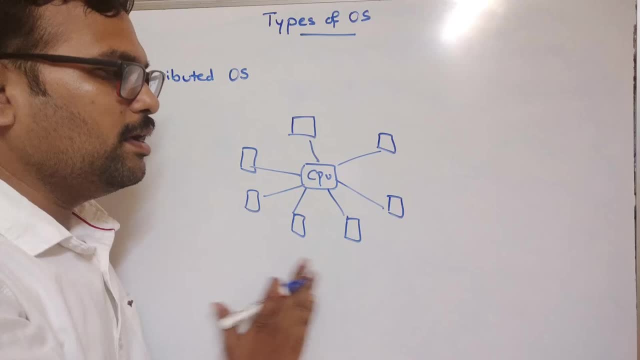 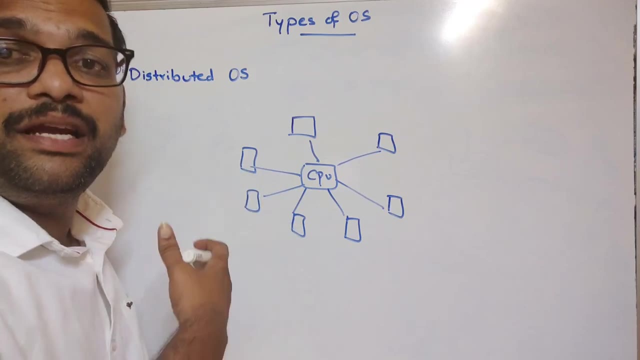 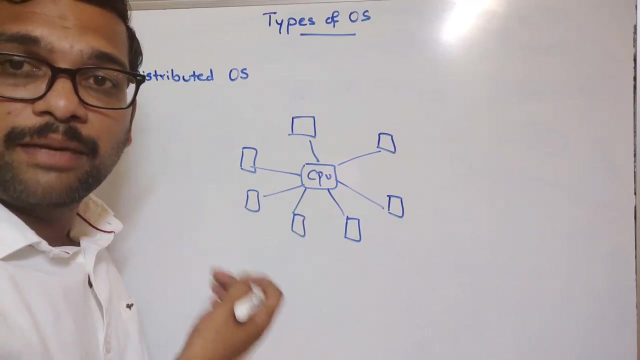 if any one fails, automatically, the remaining processors will be executed. okay, there will be no much impact on that. so the processes, the jobs, will be distributed. the processes will be distributed right throughout the network, throughout the network. so there should be some connection connection between all the networks and this. the jobs will be shared between all the systems of the. 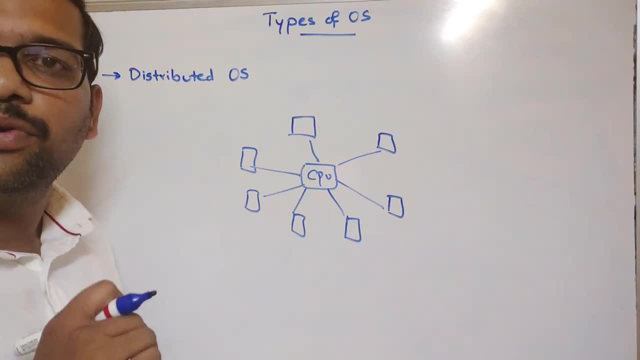 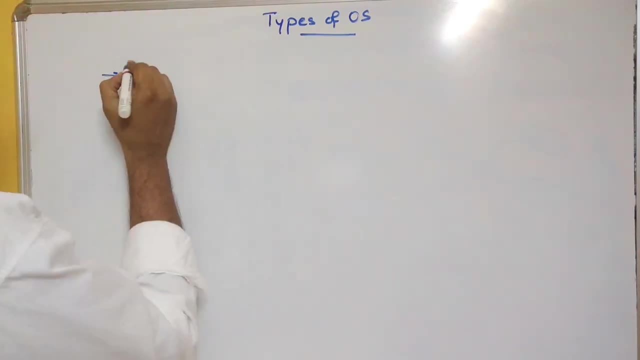 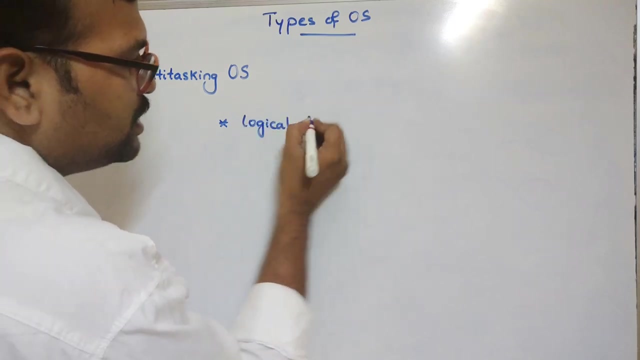 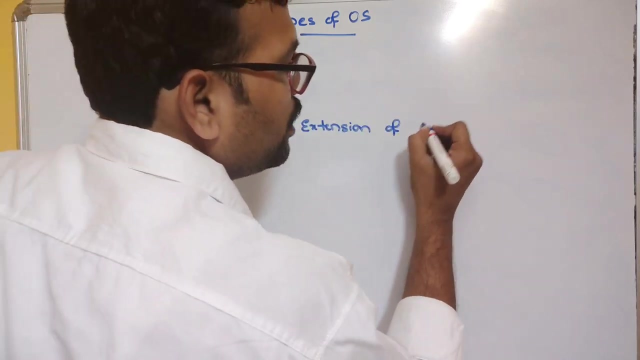 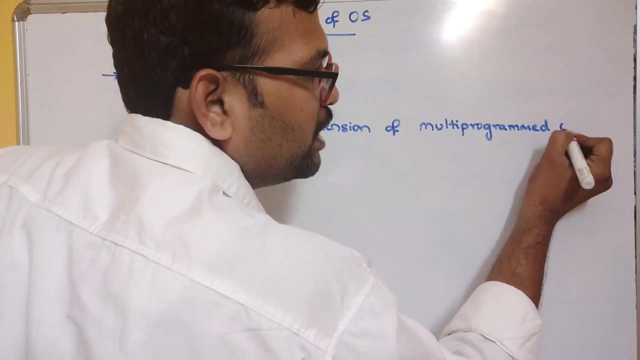 network. so this type of operating system, we call it as a distributed operating system, and the next one is multitasking, multitasking operating system. so it is nothing but logical extension, logical extension of multi programmed, multi programmed operating system. so here also multiple tasks will be given to the same CPU. okay, multiple tasks will be. 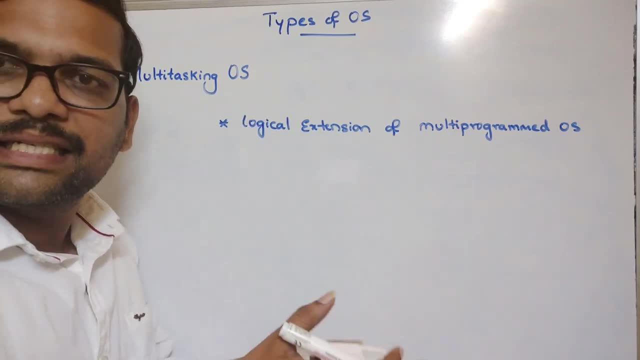 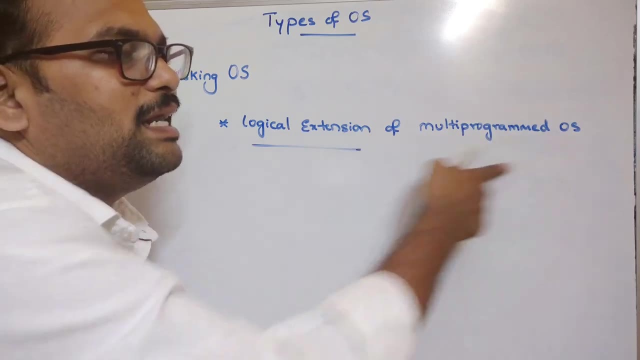 given to the same CPU, so it will be executing the multiple task. so the here also there will be no CPU ideal state, okay. so that's why we call it as a logical extension of of multi-programmed operating system, Next time-sharing operating system. 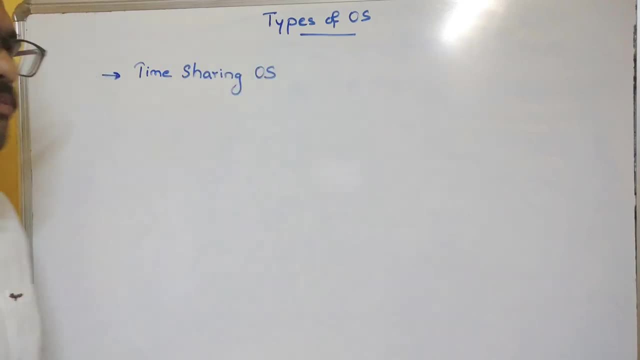 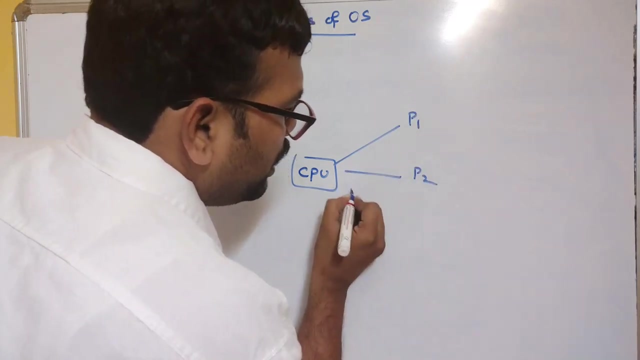 Time-sharing operating system. So in this time-sharing operating system- so the name itself indicates some time will be given for each and every process. Okay, So for example, CPU need to execute three processes, some P1, P2, and some P3.. 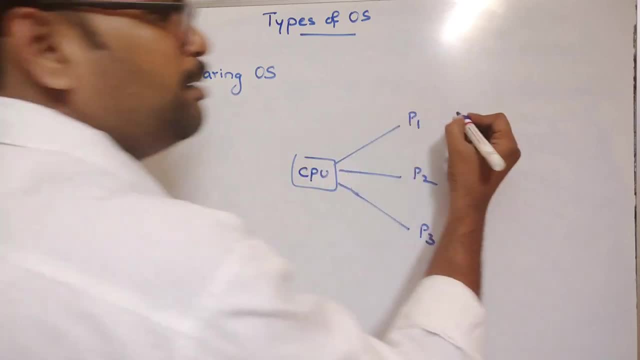 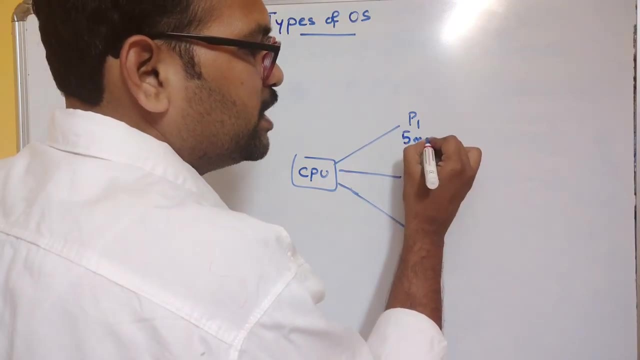 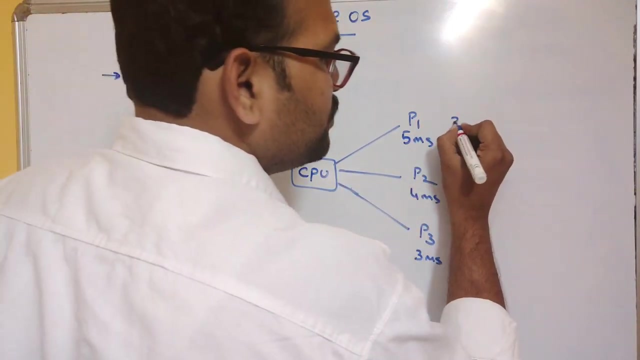 So it will allocate some time to this one. So let it be the P1 should execute. I mean, it requires some five milliseconds to execute and it is four milliseconds to execute. It is some three milliseconds to execute, So CPU allocates some three milliseconds for each. 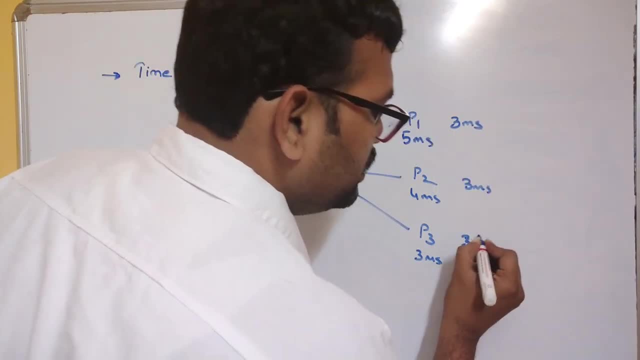 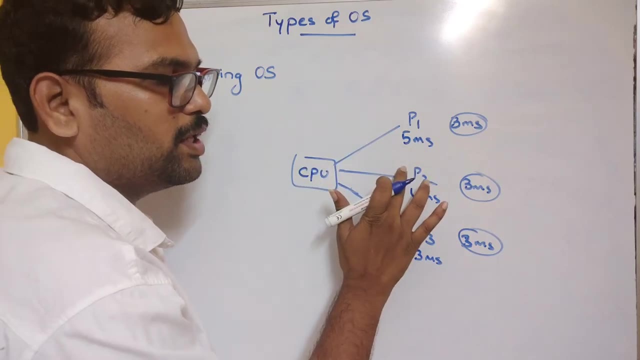 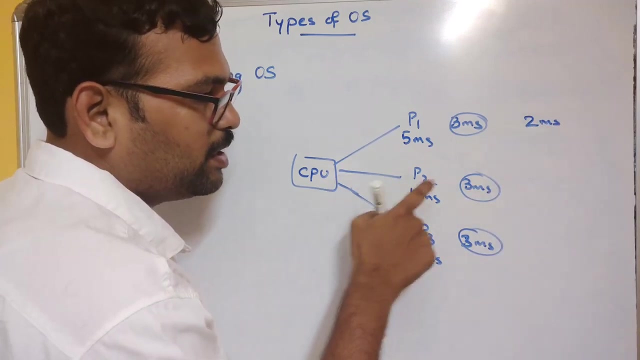 process. Okay, Okay, Three milliseconds for each process, Right, Equal distribution. So after three milliseconds, automatically the CPU will be given to the P2.. So here the remaining is two milliseconds. Okay, And here, whenever the P2 comes into the processor, it will execute three milliseconds. 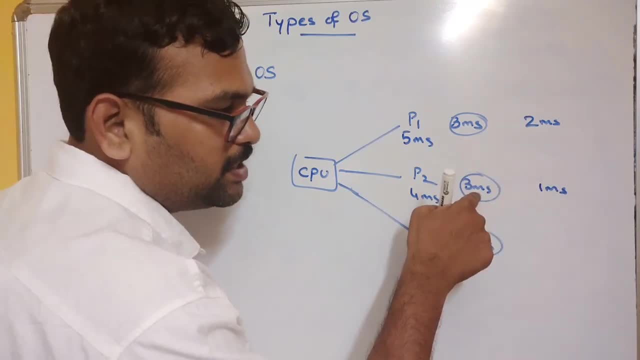 and only one millisecond is required. And again after three milliseconds. again, the CPU will be given to the P3, the process: Okay, The CPU will be given to the P3 to read: executed. Okay, So P3 will be screened in this way. Okay, Okay, Okay, bet, in that way. 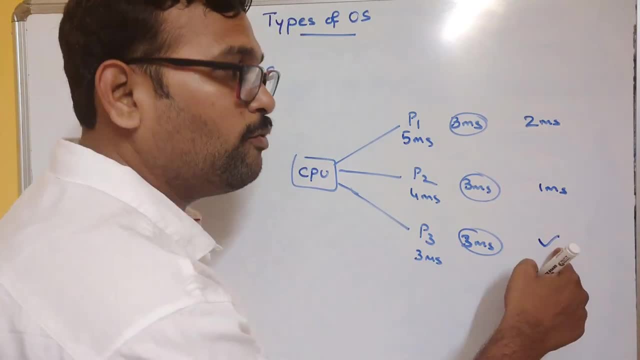 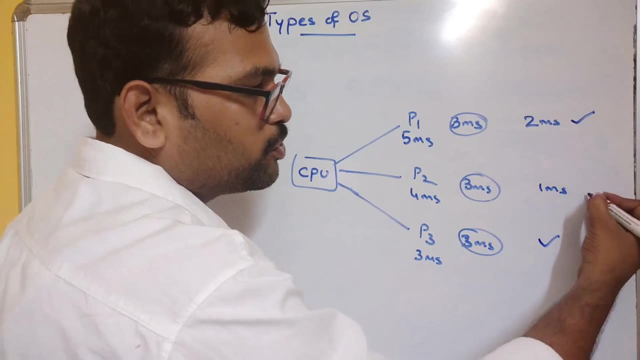 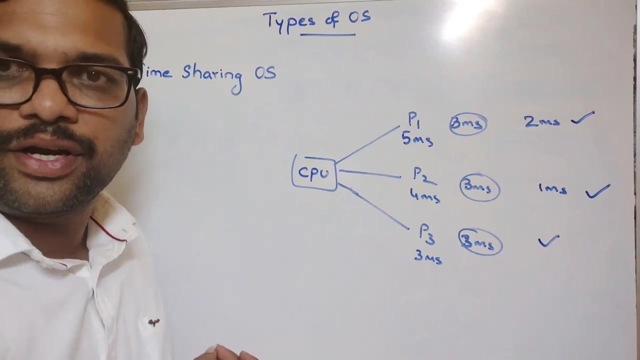 So P3 will be executed 3 times. so it will complete and once again it will come to the process 1 and it will execute this one and again. after completion of P1 it moves to the P2 right. So like this, some sort of time will be given for each process to get executed, right. 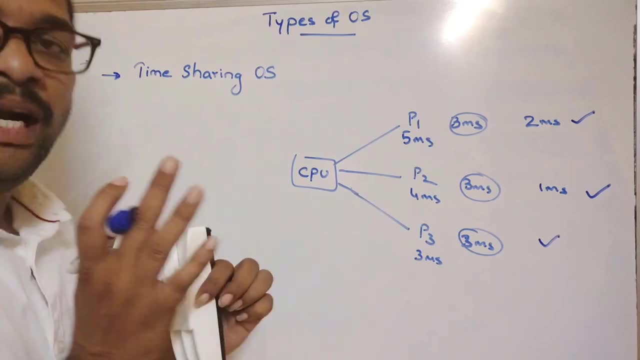 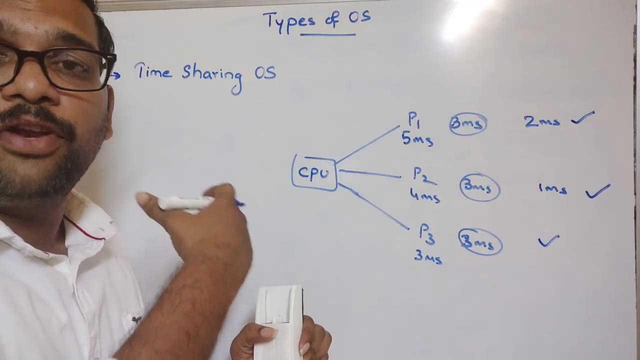 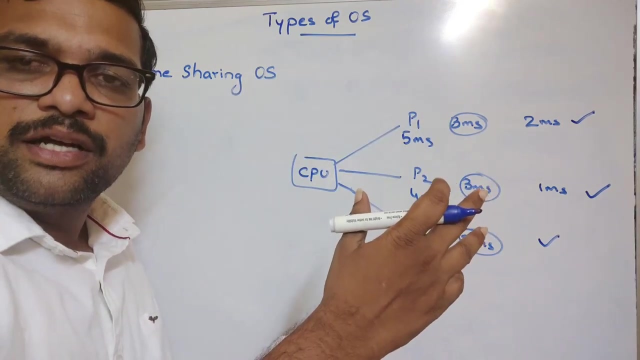 So here there is a difference between a multi-programmed and the time sharing. So in the multi-program the system will be divided. that means the system will be allocated to the processor based upon the Ivo operations. If P1 gets the Ivo operations requires Ipo operations. so instead of maintaining the CPU, 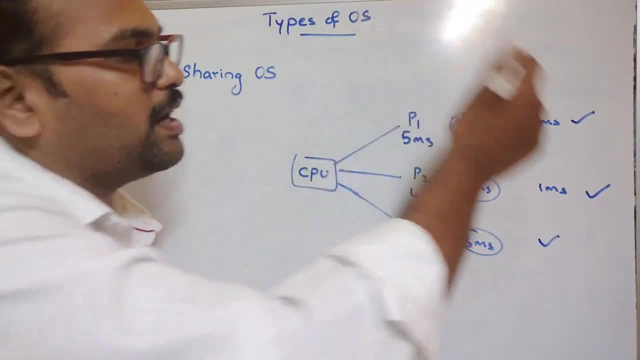 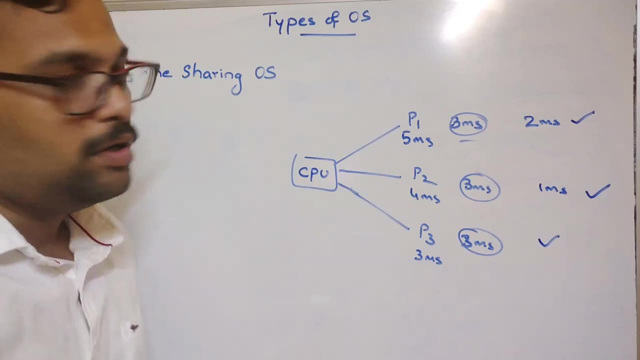 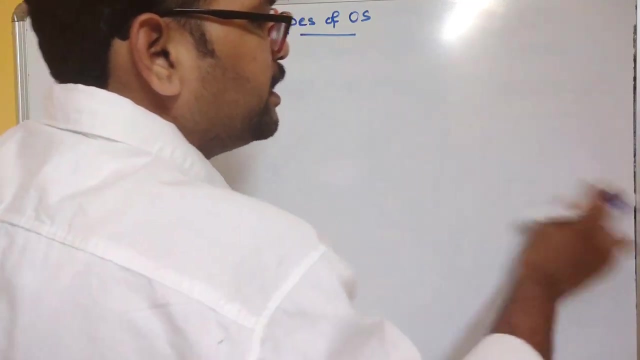 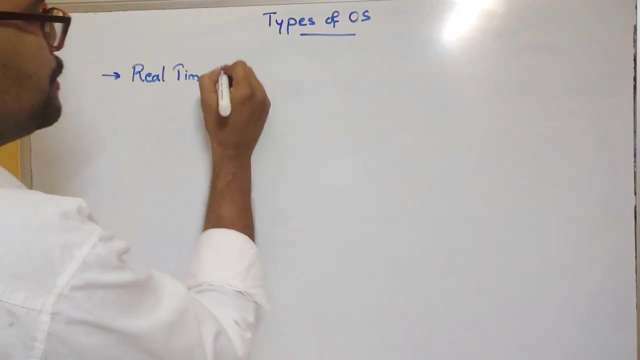 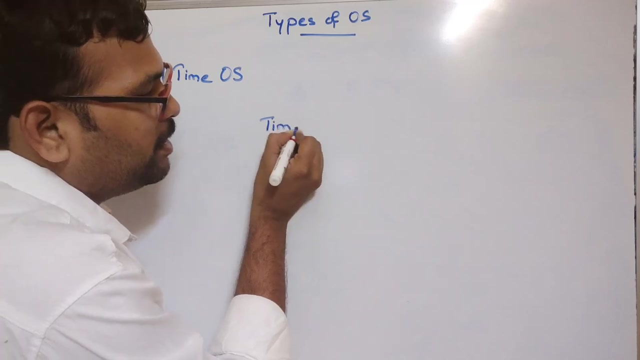 ideal, it will move to the P2, but here, after every given time, the CPU will be given to the next processes. okay, So this is the time sharing operating system and the next one is a real-time operating system. Real-time operating system, So in this real-time operating system, so we will be having some time limit and within 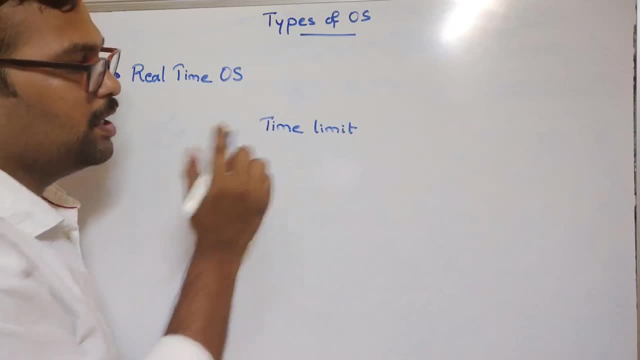 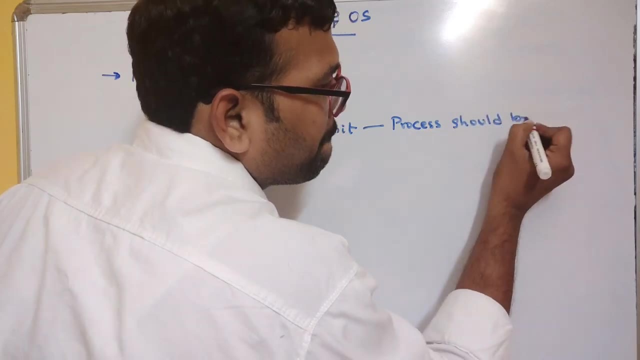 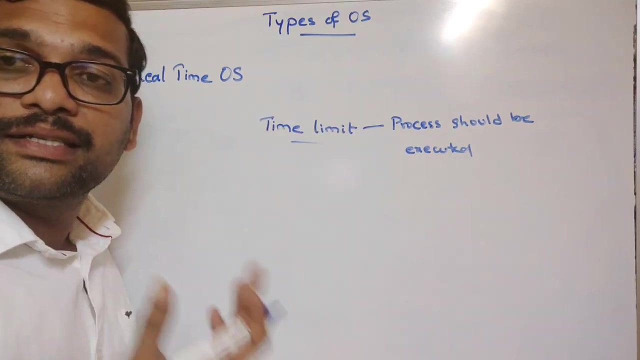 the time limit only. the process should be executed. okay, So the process should be executed within the time limit. Process should be executed within the time limit. So if it exits automatically, we will get some error. okay, So this. this is a special type of operating system which gives the time limit for each. 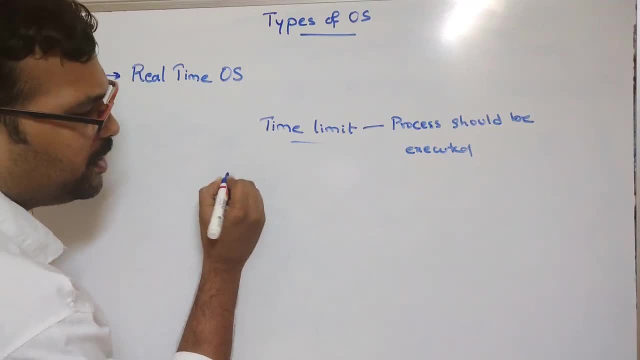 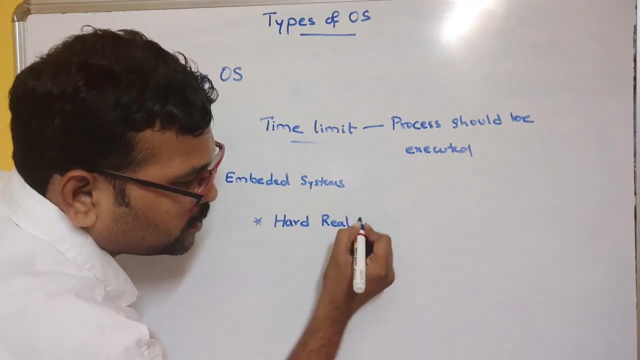 process to be get executed. So usually it will be used for embedded systems. embedded systems, okay, embedded systems, and here there are two types of real-time operating systems. One is hard real-time operating system- hard real-time operating system- and soft real-time operating system. 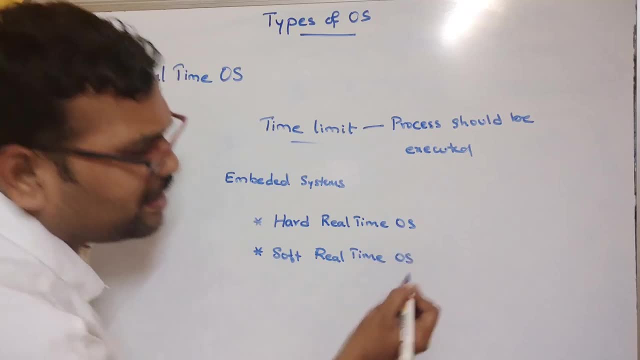 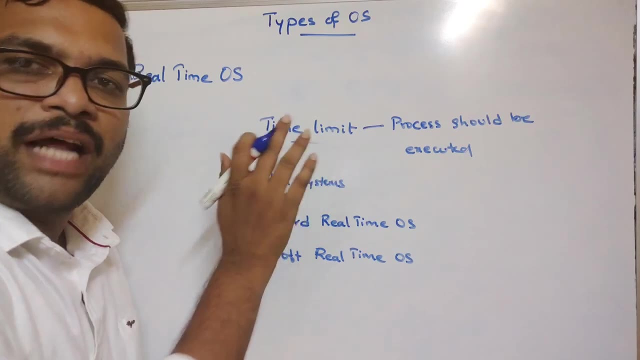 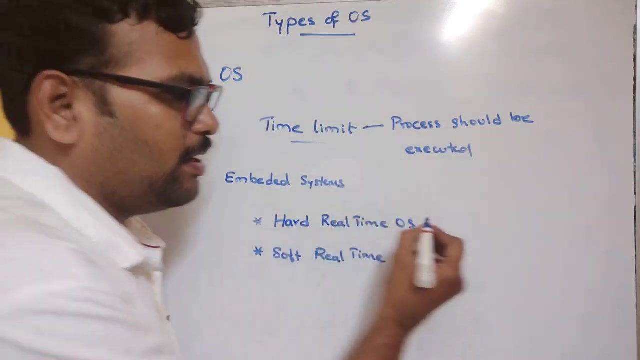 So here there is a slight difference between hard and soft. so in both the cases the system will give some time limit and within the time limit we have to complete the process. So if the time limit exits in this hard, hard, real-time, automatically it leads to the failure. 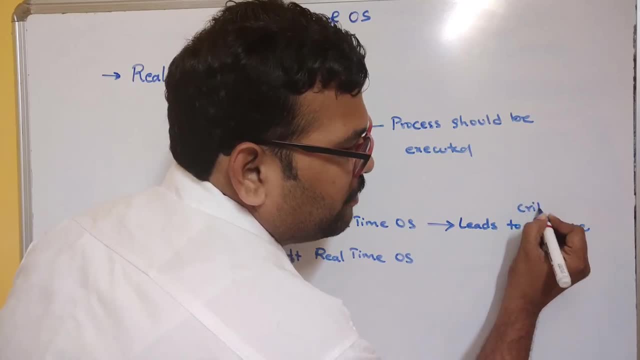 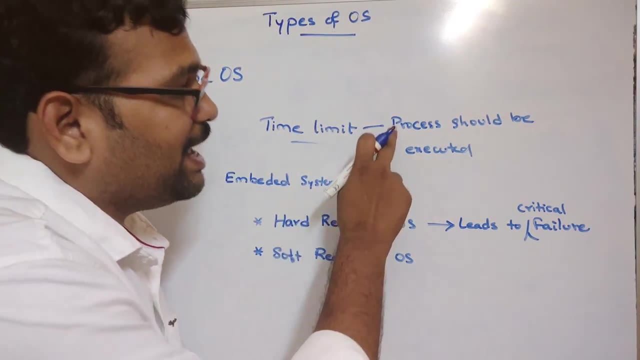 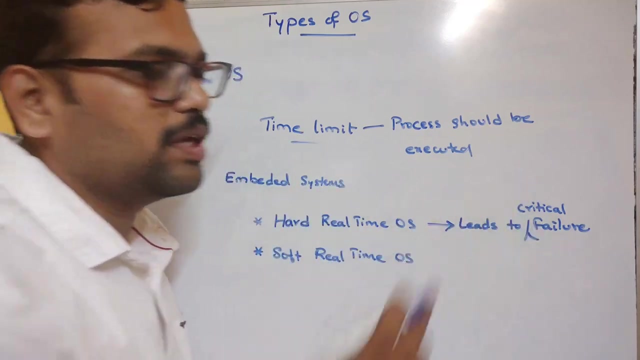 system failure, all critical failures, okay, critical failures, or a device or a system, whatever it may be. So when the process- exec- I mean- exceeds the time limit, okay, the execution of process exceeds the time limit, automatically it leads to the critical failure. So that's called a hard, real-time operating system.